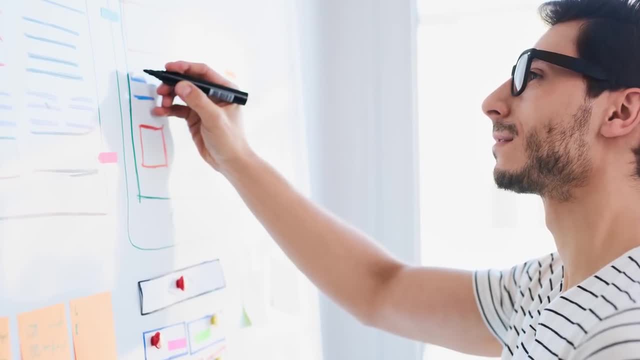 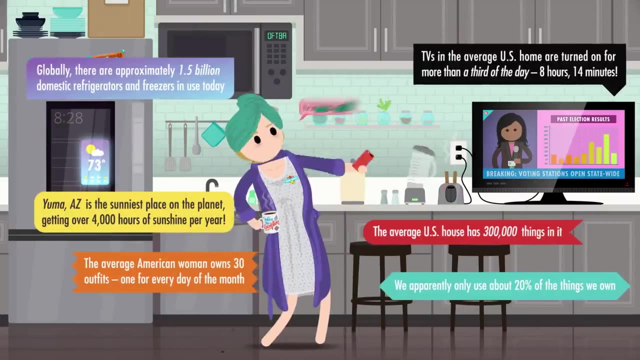 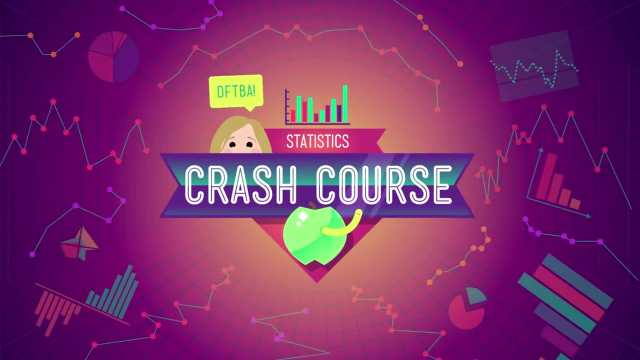 has helped companies make marketing decisions, like which color to use on their website, and it's helped researchers quantify their results in scientific studies. Today we're going to talk about it First. you may have noticed that so far, when we talk about the math of Bayes' theorem, 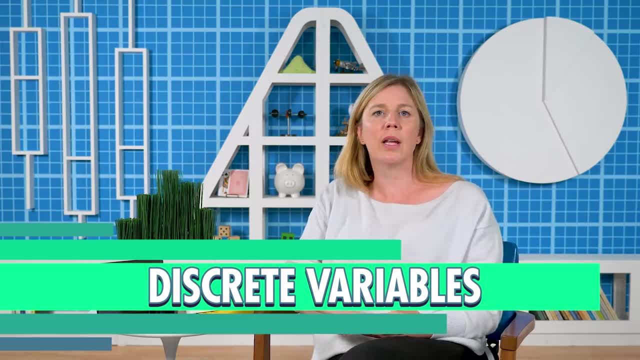 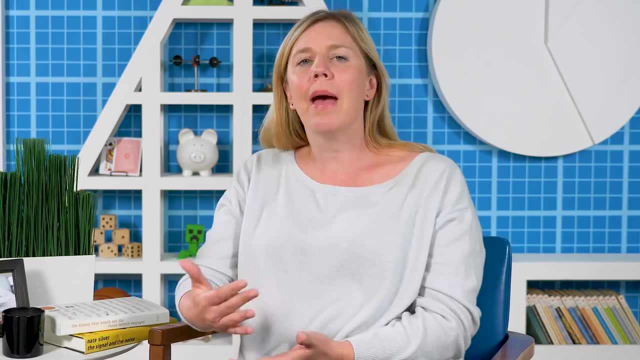 we've been using discrete variables like whether or not you're a Star Wars fan or whether or not you have a disease, But Bayes' theorem can help us update beliefs that involve continuous variables too. The math of Bayes' theorem with a continuous variable is a bit more complicated than in. 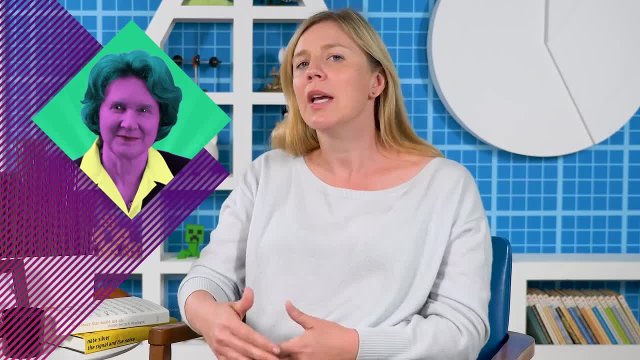 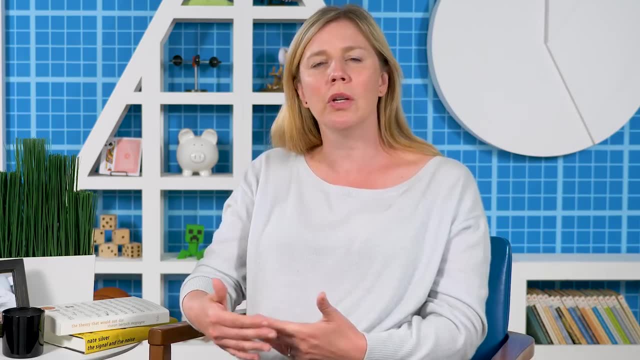 the discrete case. Science writer Sharon Birch-McGrain called it a theorem in want of a computer. In fact, for much of the 20th century, scientists and statisticians who wanted to use Bayes were limited in their ability to do so by a lack of computational power. 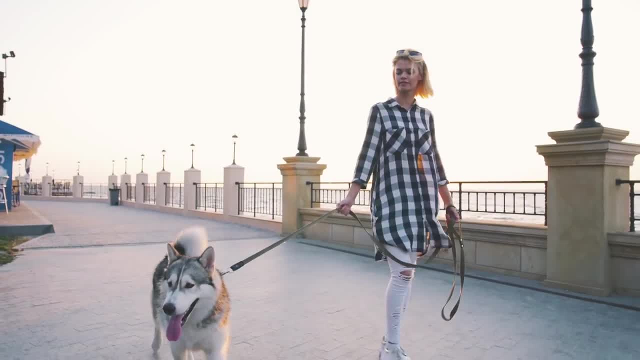 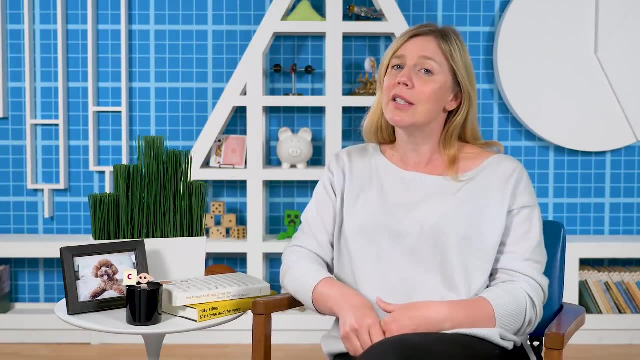 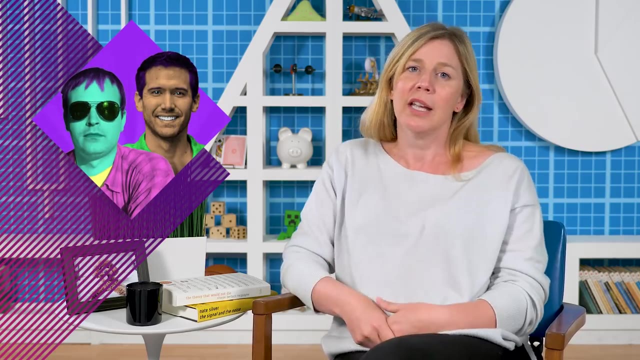 But we still want answers to those more complicated problems. Sometimes we want to know whether dogs who are walked regularly are less likely to damage furniture, or whether house elves have lower intelligence than wizards, which is an example of Bayesian hypothesis testing from a Harry Potter-themed article by Etz and Vanderkerkof. 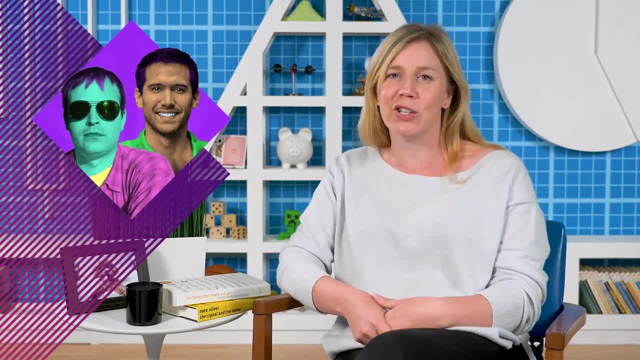 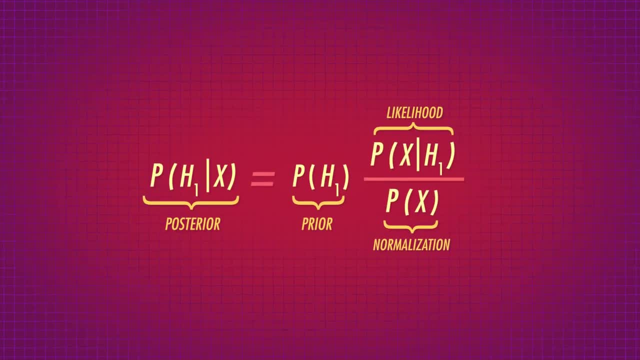 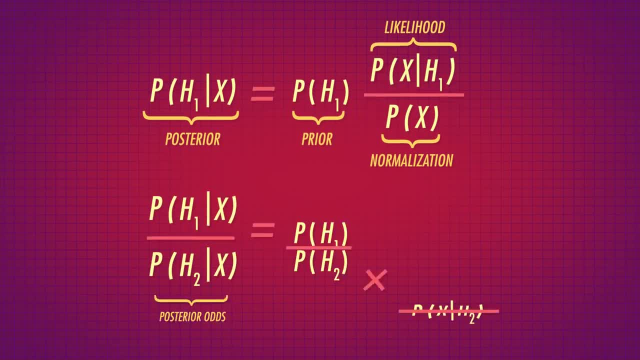 We can't do anything about it. We can't do anything about it. The way we update our prior beliefs is the way we estimate it with the likelihood of our evidence. This is called the Bayes factor when comparing two models, Once we've updated. 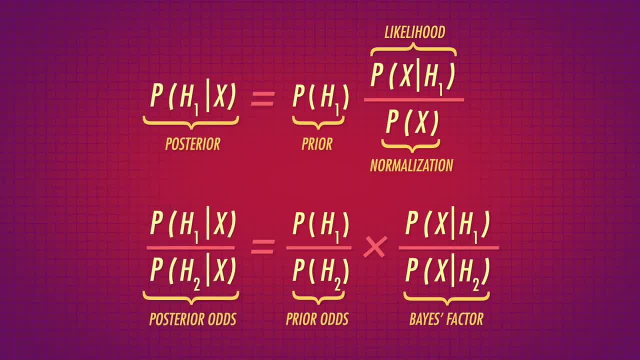 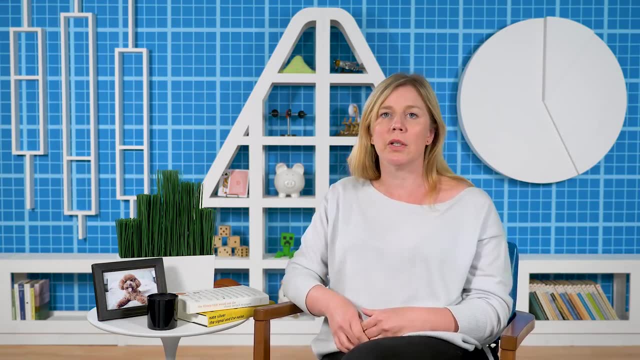 our new beliefs are called our posterior beliefs. If we're comparing two models, they're called our posterior odds. But instead of simple discrete probabilities we have probability distributions. For example, let's look at the ever-present problem of whether or not a coin is biased. 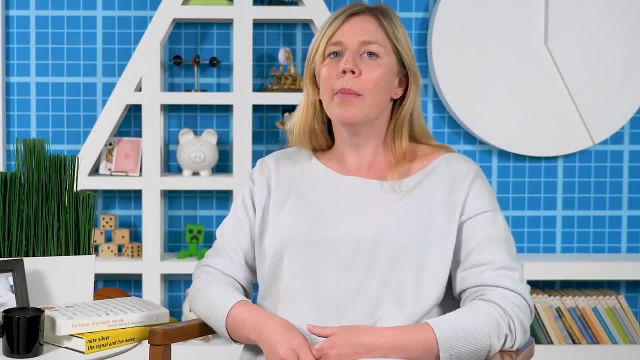 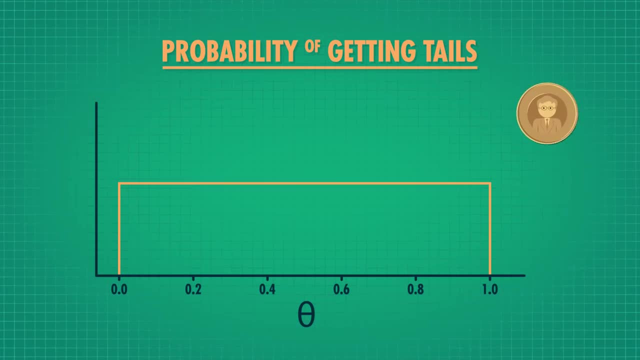 Before you start your experiment to test the fairness of your coin, you decide that you know almost nothing about whether or not it's biased. So your prior probability of getting tails is a uniform distribution between 0, never tails, and 1, always tails. 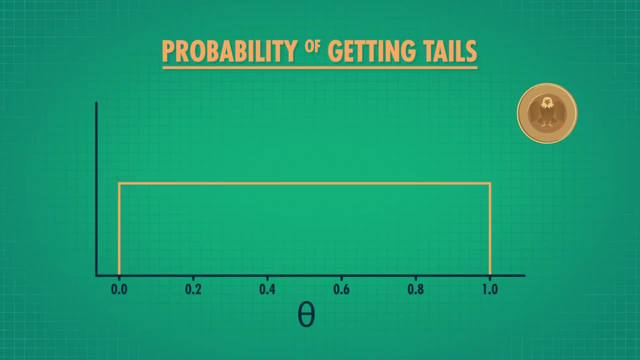 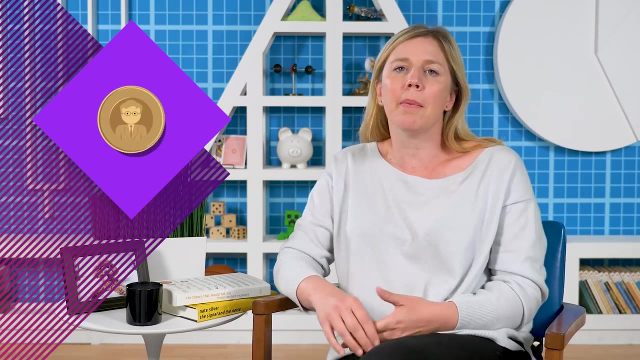 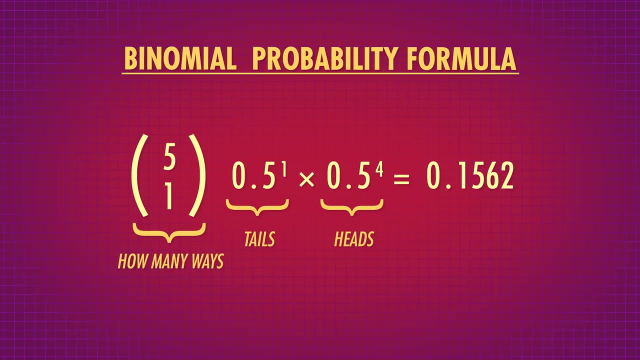 You consider all probabilities of getting tails- we'll call that theta- equally likely. You have a friend: flip the coin in question 5 times and they get 1 tail, which seems unlikely, though not impossible for a fair coin. Using the binomial probability formula, we know that the probability of this happening 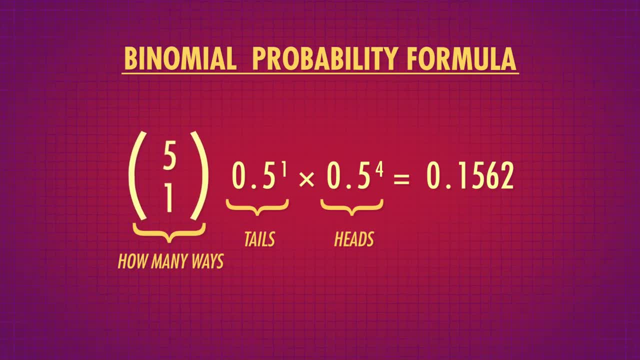 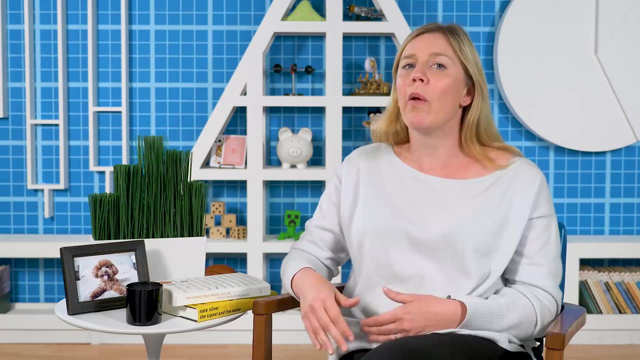 with a fair coin is about 16%. Note this new notation: for 5, choose 1,. you're most likely to see it like this in the stats world. So how does this evidence update your belief about what the real probability of getting a tail is for this coin? 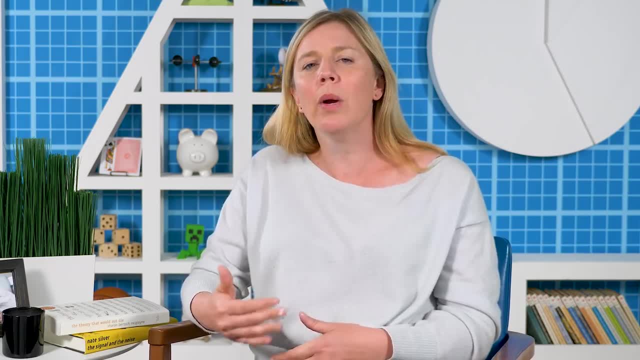 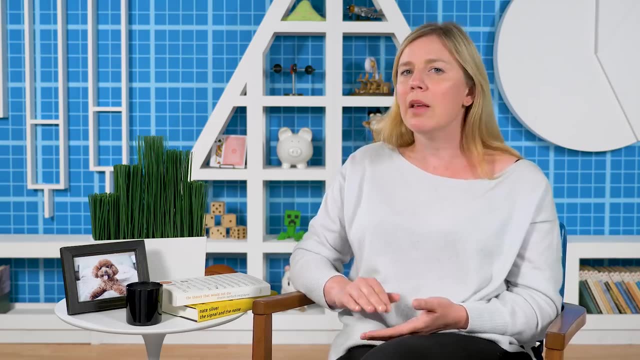 Before we show the Bayesian calculation, let's take a moment to figure out what we think. without the math- Since we saw at least one head and one tails- we can rule out both the probabilities 0 and 1.. And we think that the probabilities very close to 0 and 1 are unlikely too, because it'd 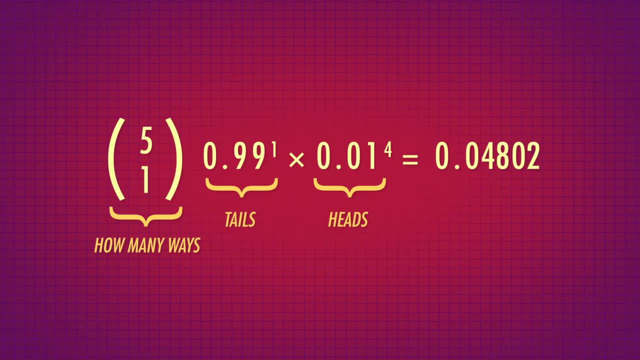 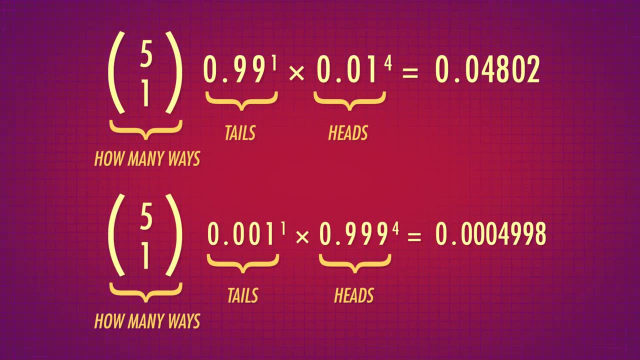 be really rare to see only one tail if the probability of tails were .99.. And similarly rare to see a tail at all if the probability were 0.001.. Now we can do the Bayesian calculation and see if it matches our intuition. Here's Bayes' theorem. but for this continuous problem. 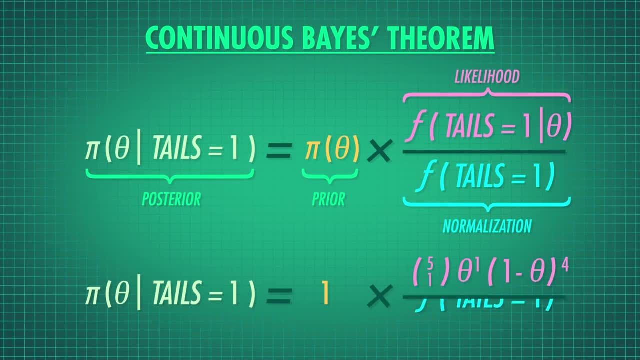 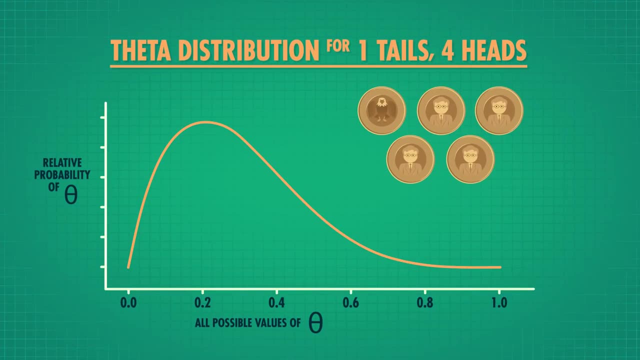 We won't get too stuck on the math here, but we can see that this is the same old Bayes' theorem that we've seen before, just continuous. When we plug in this formula to a graphing program to show our posterior, it looks like. 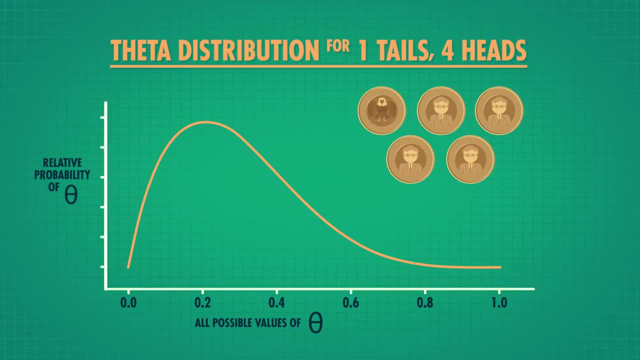 this: The Y axis tells us the relative probability of a theta. For this case, theta tells us the probability of a theta and in this case, theta is the probability of a theta- the probability of getting tails. and the x-axis shows us all the possible values of. 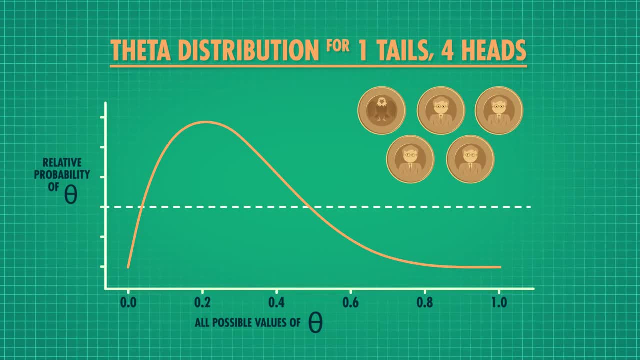 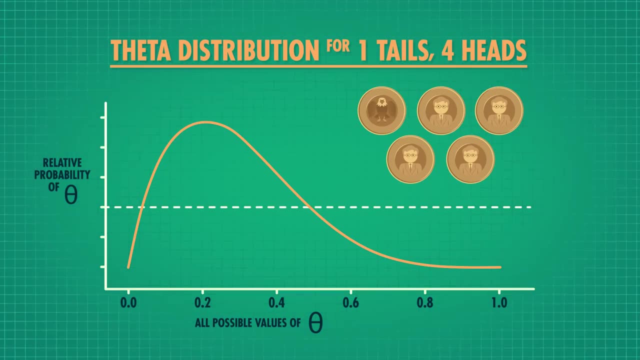 theta between 0 and 1.. We can see that we took our prior distribution, the dotted line, and updated it using the likelihood of the data, which told us the probability of getting 1 out of 5 tails for every potential probability of getting tails that a coin could have. 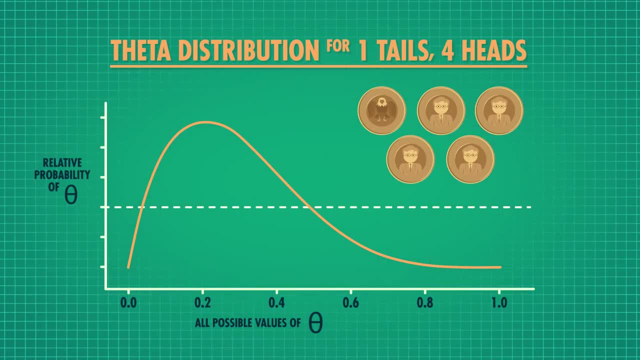 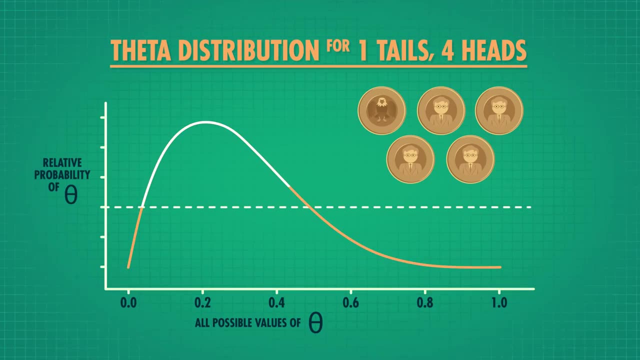 Once we updated our prior beliefs about which probabilities are the most likely. our posterior beliefs are represented like this: the solid line, Anything on the curve that is above the dotted prior line represents a theta that became more likely after we saw the data, And anything on the curve that is below the dotted line is a theta that became less likely. 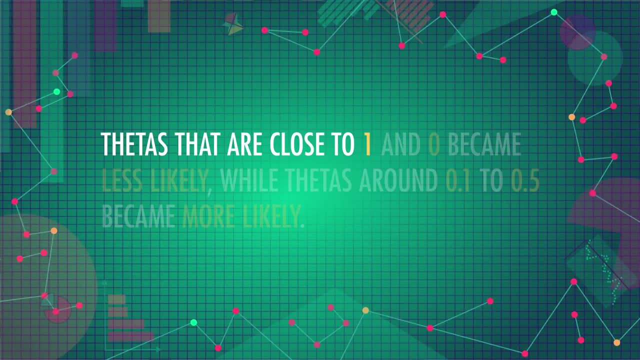 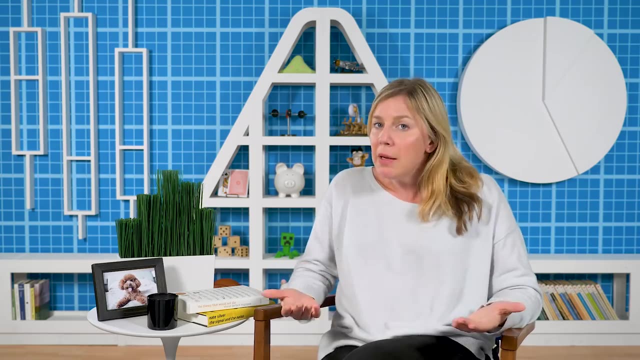 And this matches our intuition- Thetas that are close to 1 and 0 became less likely, while thetas around 0.1 to 0.5 became more likely. So maybe we have a fair coin here, but it seems more likely that it's biased. 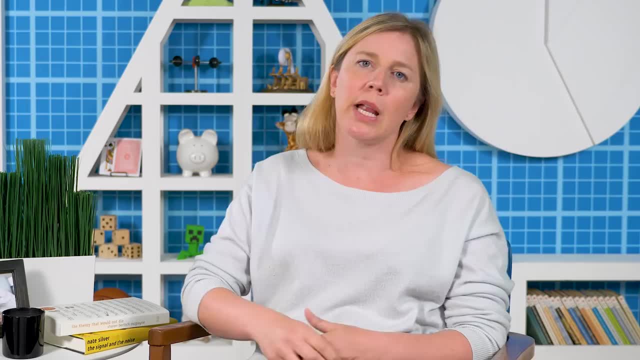 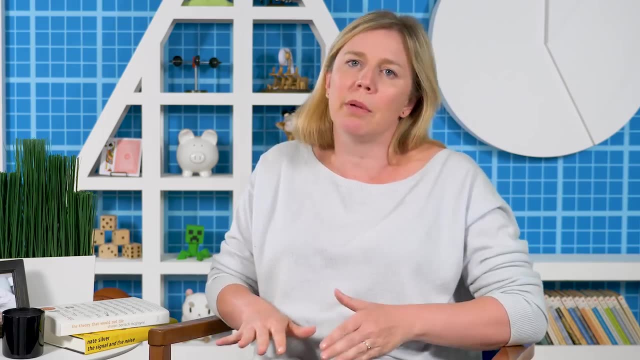 This is like Bayes, because it allows them to take into account previous knowledge and expert opinion when they make their calculations. Let's look at how a business might use Bayesian inference. We'll keep the math to a minimum here, but if you're interested in learning more, you. 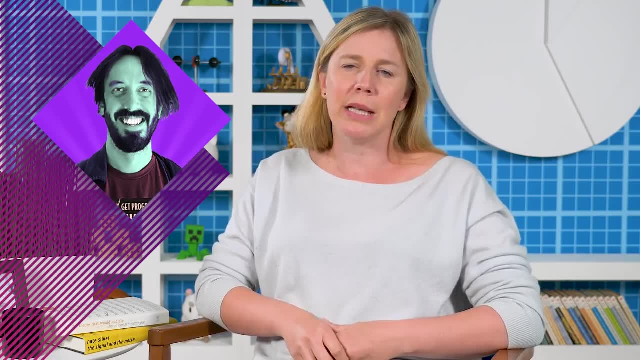 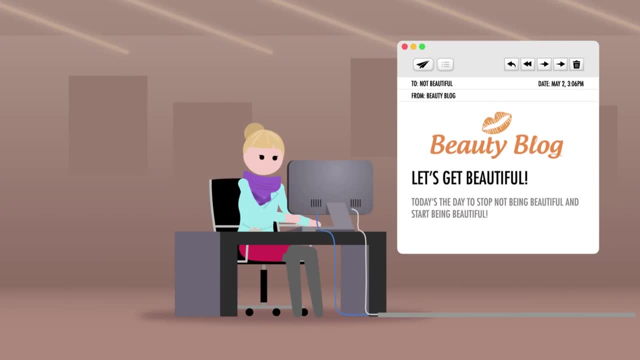 can check out this awesome blog post by Will Kurt on countbayseycom, which we based our next example on, And the link's in the description Say: you're a beauty blogger and you send out weekly emails encouraging your followers to read your latest blog post. 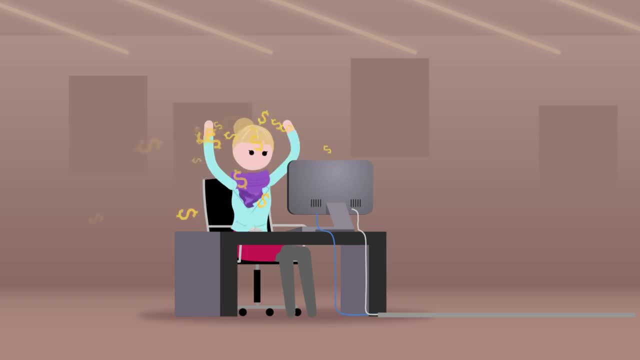 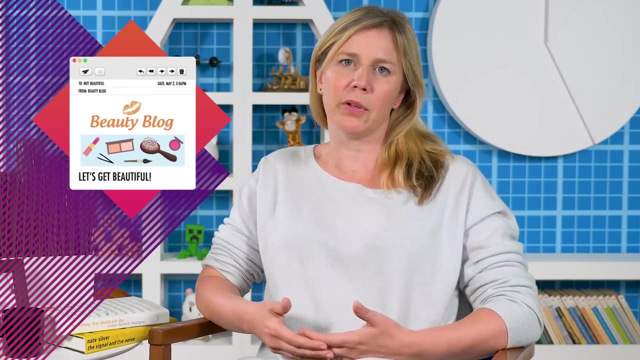 The more people who click, the more money you make, And so you want the most out of it, The most clickable emails ever. Your friend, who's also in the blogging business, told you that adding a picture at the top of your email gets more people to click. 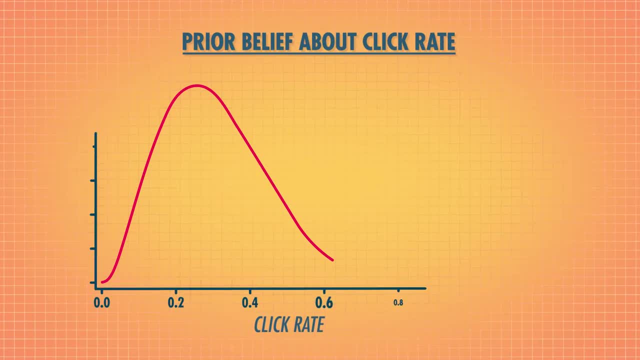 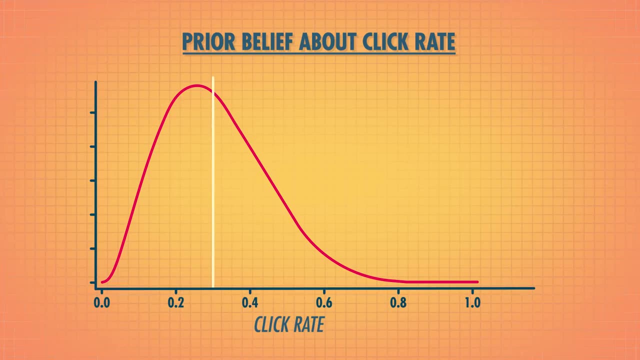 But you want to test that idea out with your own readers. Normally your click rate is around 30%, so you decide to represent your prior beliefs about your true click rate using this function. Values around 30% are most likely, but it's possible your true click rates are higher. 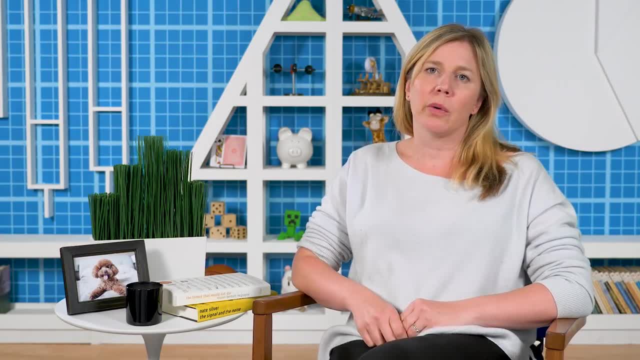 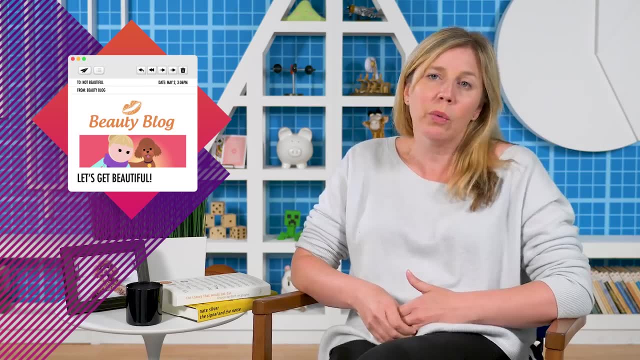 or lower than that. You randomly select 300 of your followers to be part of your experiment, often called an A-B test in the business world, And send half the email with a cute picture of you with your poodle ginger, as well as. 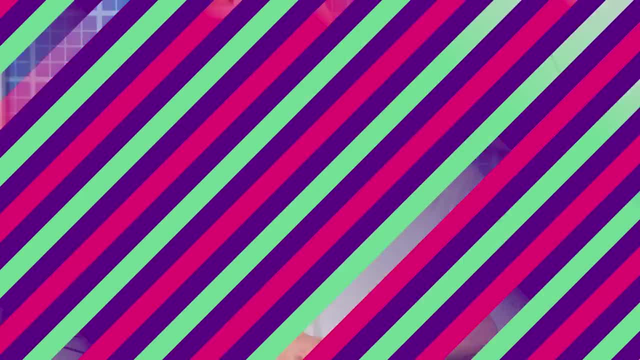 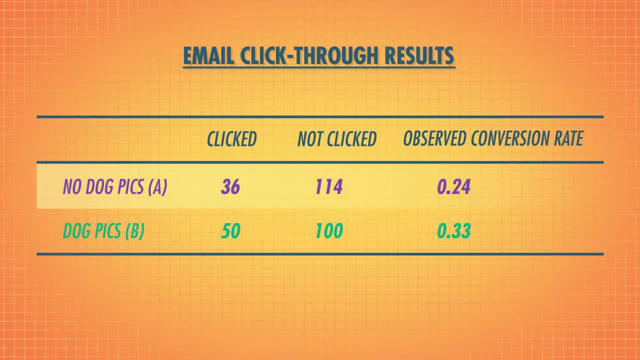 the normal content. The other half gets your standard picture-less email. You anxiously await the results and three days later you have them. You can use the new information you have about your two emails to update your original beliefs about your click rate. 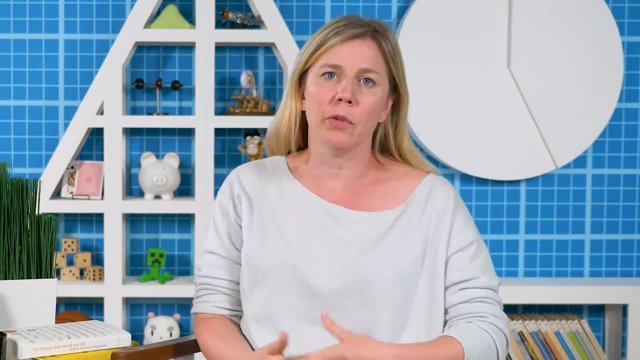 Since the two groups were the same before you assigned them to get either email no dog pictures or with dog pictures, you use the same prior for both groups. Once you've incorporated this new evidence, your posterior district will be able to use the same prior for both groups. 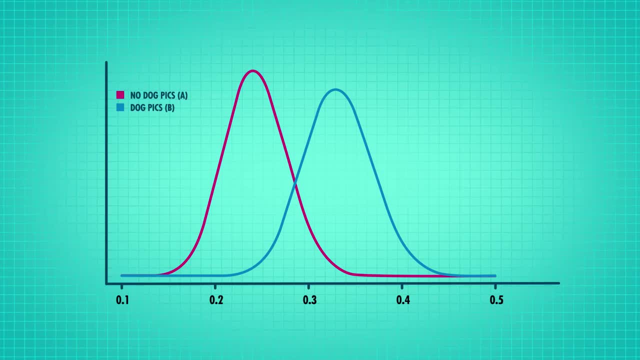 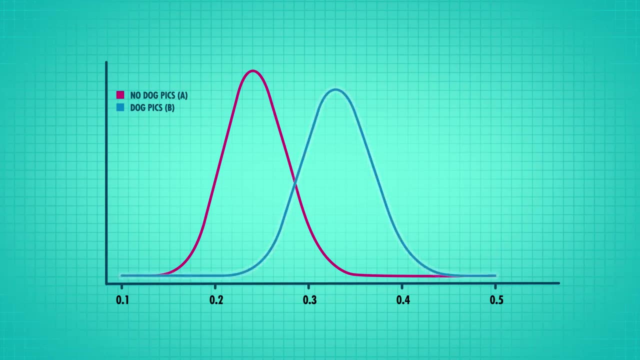 Once you've incorporated this new evidence, your posterior district will be able to use the same prior for both groups And they tell you how likely each click rate is. under your new posterior beliefs about each group, It looks like the group with pictures is likely to have a higher click rate, but you can't. 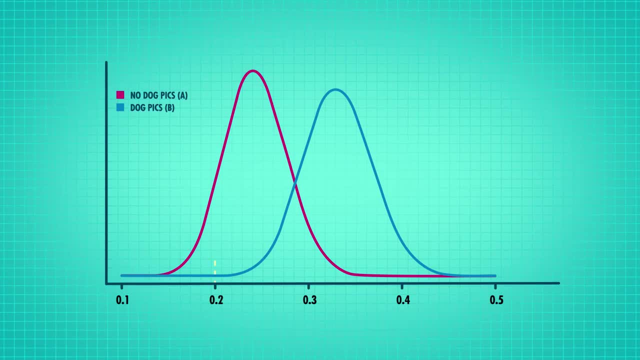 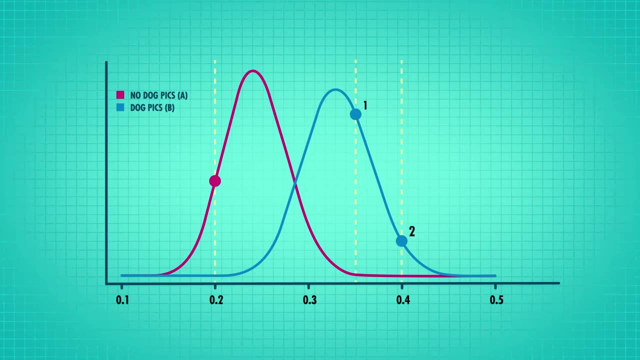 know for sure. One way to get more information to make your decision is to randomly simulate a bunch of samples, one at a time. The samples come from each of your two posterior distributions and then you count how often the group with pictures' click rate is higher than the group that didn't get a picture. 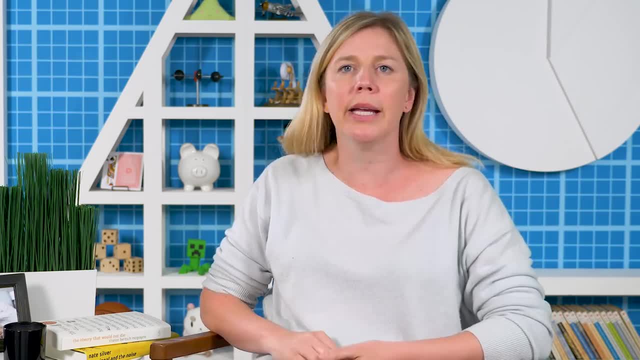 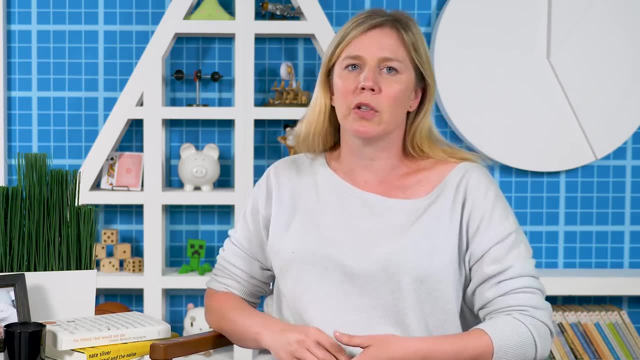 in their email. That percentage will tell you roughly how likely it is that the group that got pictures will have a higher click rate than the group who did not. You decide that if, in 70% of your simulation samples, the group with pictures has a higher 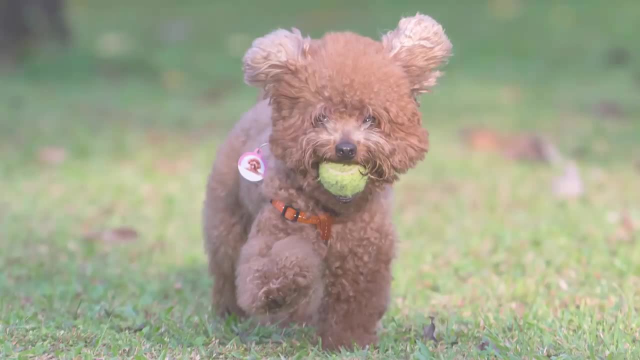 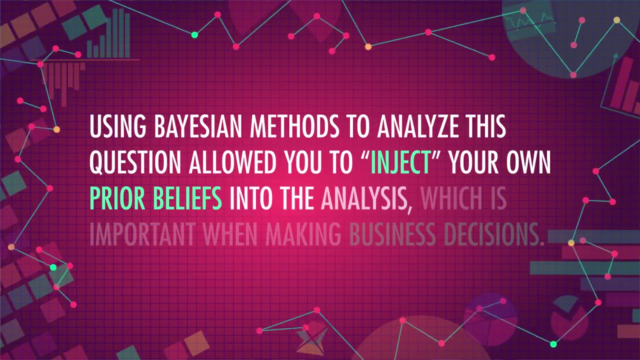 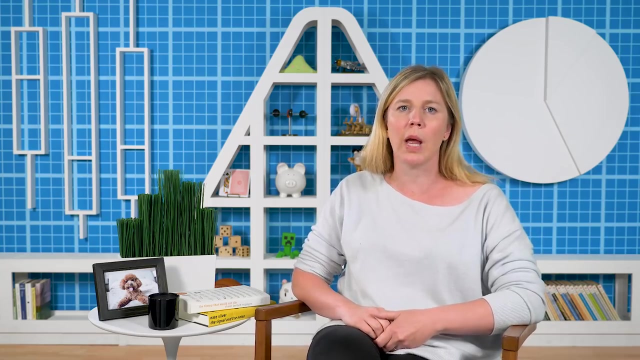 click rate, you'll include glamour shots of ginger in all your new emails. Using Bayesian methods to analyze this question allowed you to inject your own prior beliefs into the analysis, which is important when making business decisions. Businesses often want to make the best decision in the most cost-efficient way. 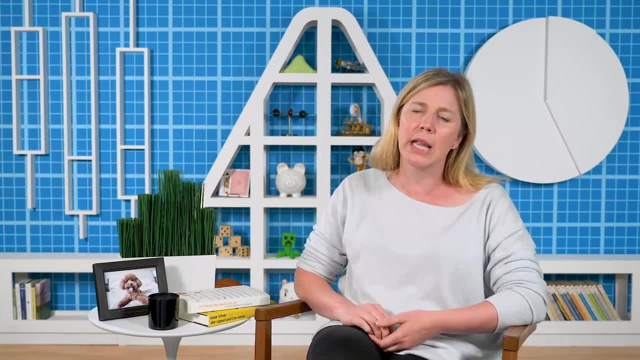 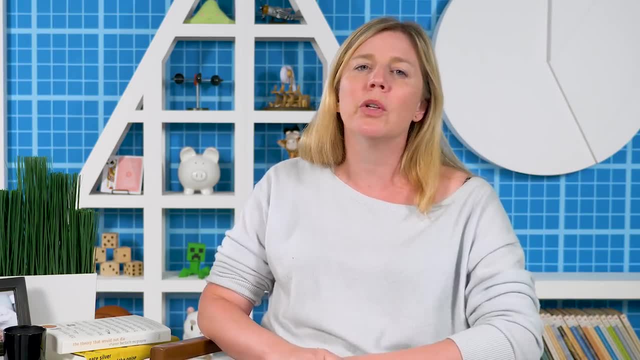 This means taking advantage of all the information they have, not only data, but prior knowledge of the field and expert opinion. Your prior knowledge about the click rate of your emails made it possible for you to start your analysis, knowing it's pretty unlikely. your click rate was very near zero. 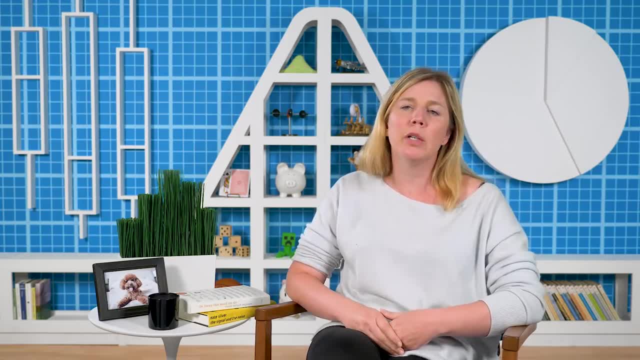 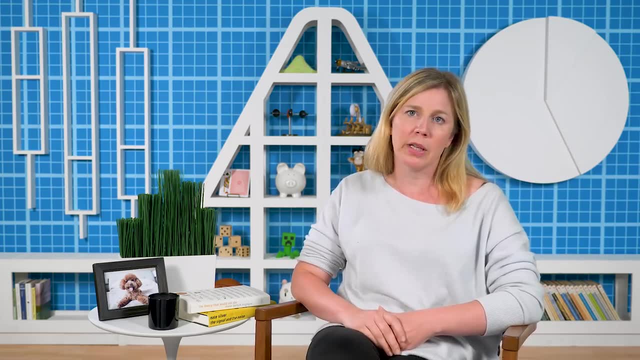 or very near one Bayesian analysis can be incredibly useful in science as well. A study on dissociative identity disorder, or DID, formerly called multiple personality disorder, looked at whether people with DID had different mental and physical disabilities. They found that people with DID had different mental and physical disabilities than people. 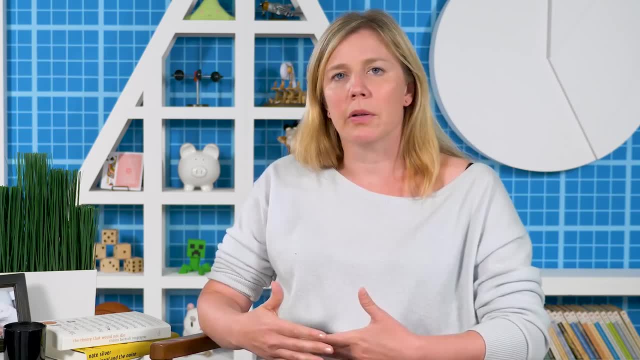 with DID had different mental and physical disabilities than people with DID had different mental and physical disabilities. They also found that people with DID had different mental and physical disabilities than people with DID. If one person had two separate personalities- Bob and Alice- researchers were interested. 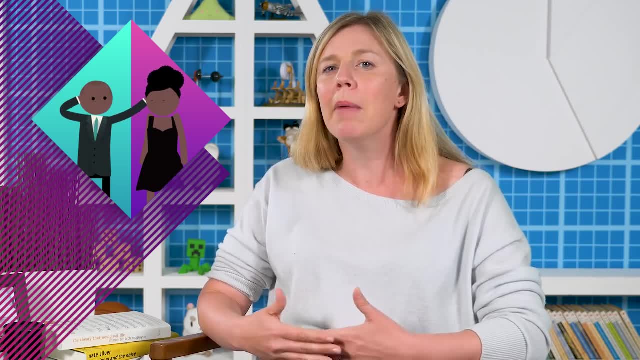 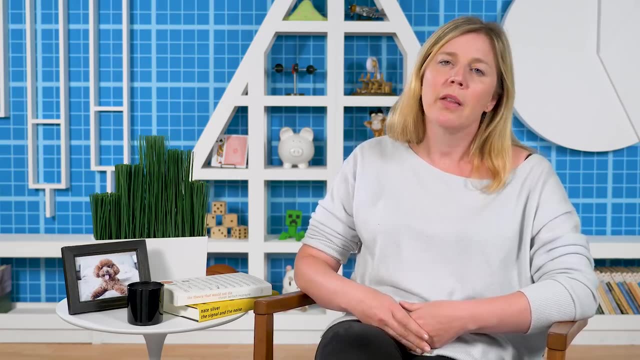 in whether something that person learned as Bob could be remembered by that person when they were Alice. In order to test this idea, participants were shown a few pictures and told a story. They then waited a little while and answered 15 multiple choice questions about the material. 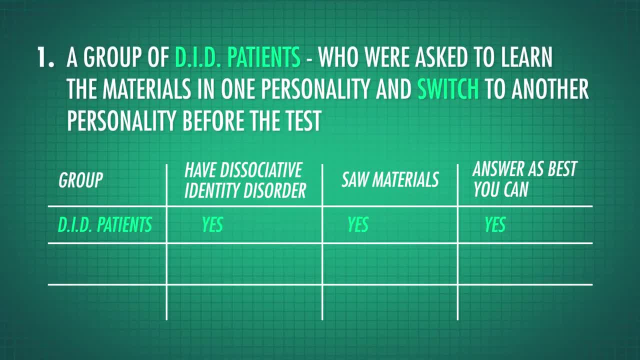 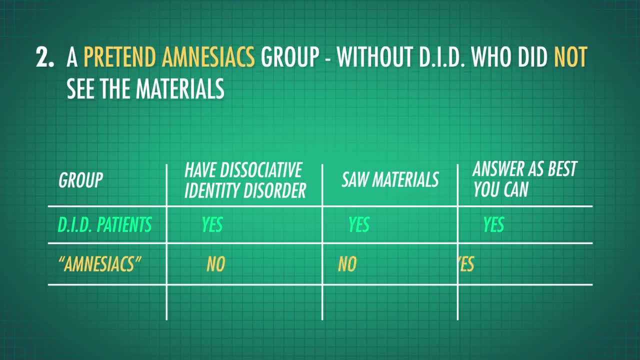 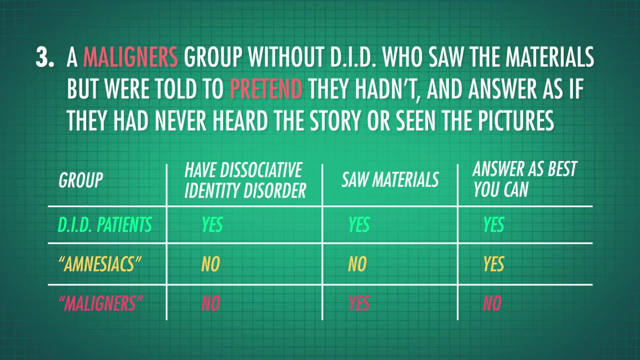 There were three different groups of participants: A group of DID patients who were asked to learn the materials in one personality and switch to another personality before the test. a pretend amnesiacs group without DID who did not see the materials. and a maligners group without DID who saw the materials but were 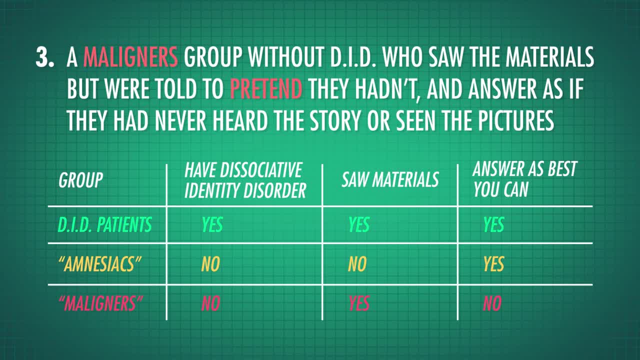 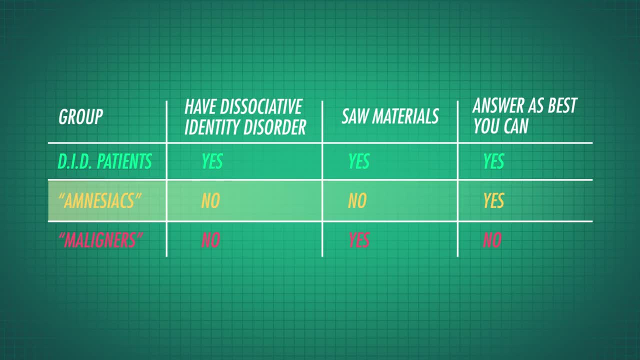 told to pretend they hadn't and answer as if they had never seen the story or seen the pictures. Researchers wanted to know whether the patients with DID, the people who had never seen the materials and the people who were pretending not to have seen the materials had the same. 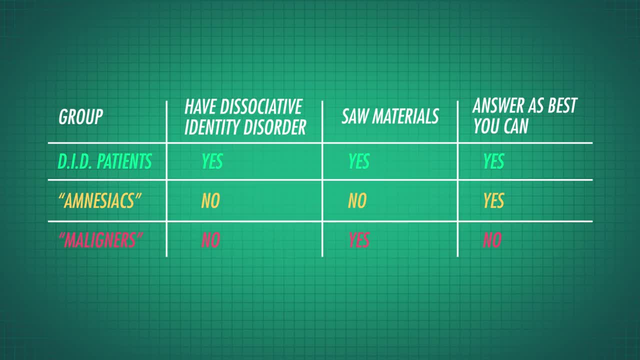 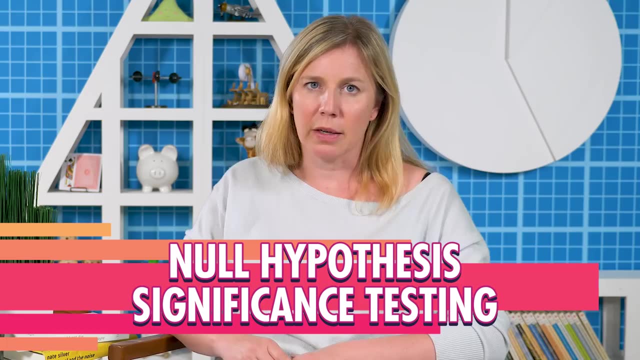 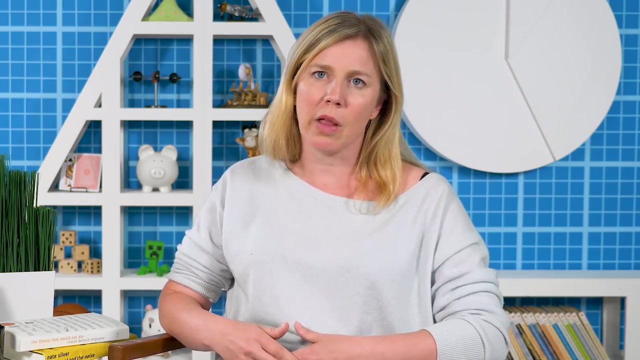 mean accuracy on the test. This would help researchers and cognitive scientists understand more about how memory works in DID patients. Using null hypothesis significance testing, researchers could try to address whether all three groups had the same mean score on the test. But even if they rejected the null hypothesis that all three groups are the same, they wouldn't. 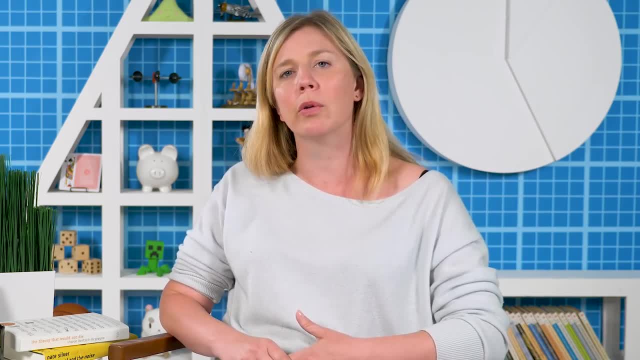 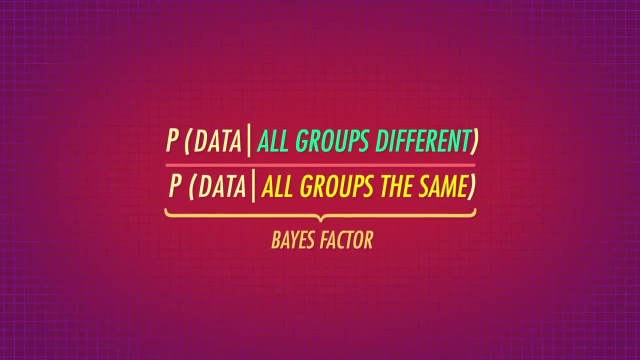 be able to say how much more likely it was that all three groups were different. Bayesian methods can tell you that, And a group of researchers did analyze the data this way and found that the Bayes factor for these models was about 4,000.. 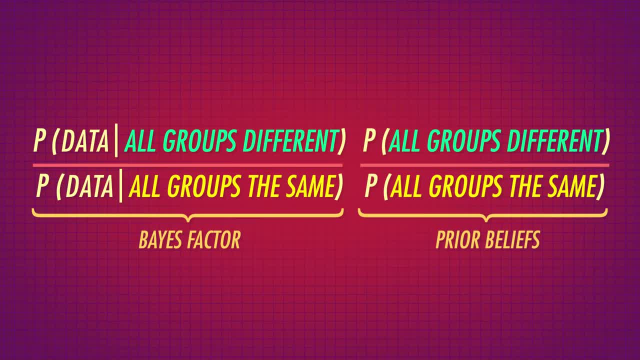 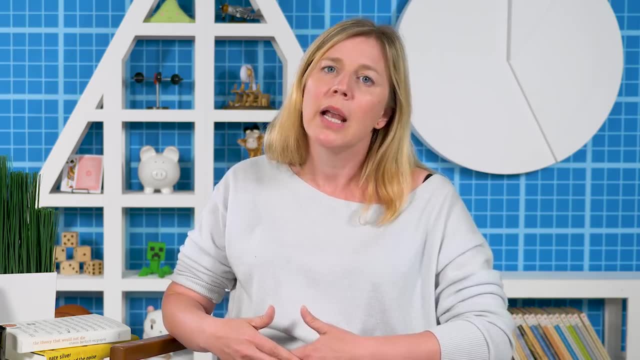 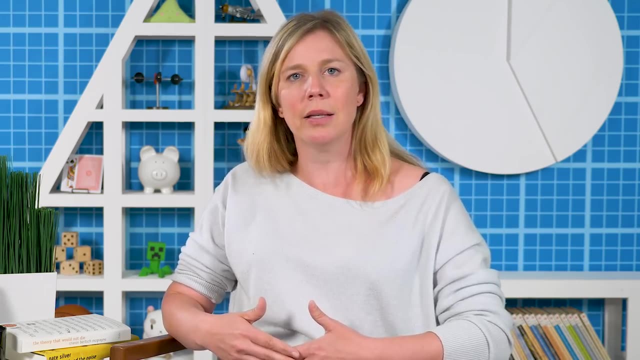 That means that the data that the researchers saw should update our beliefs by a lot. No matter what you believed beforehand, your updated beliefs will most likely reflect the fact that it's more likely that these three groups DID- patients, people who didn't see the materials and people who pretended not to see the materials- are three distinct. 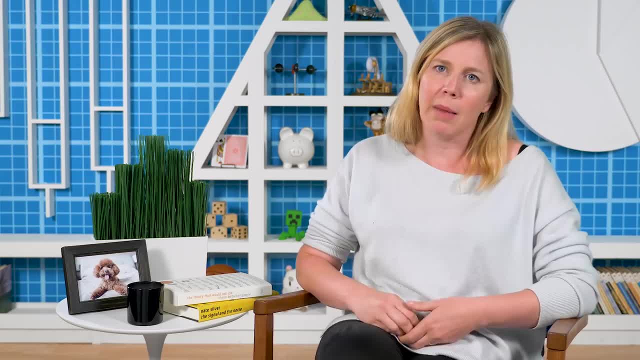 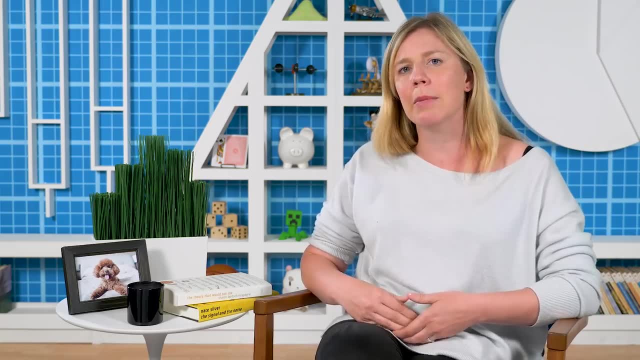 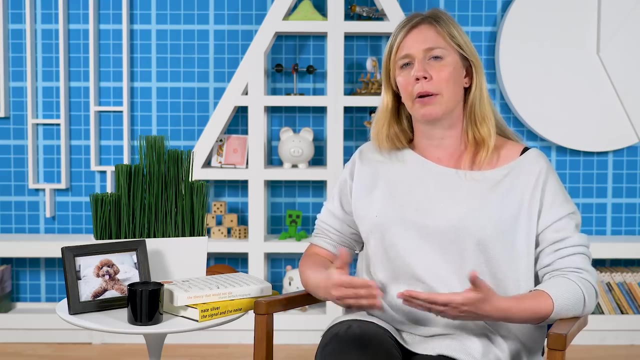 groups, And it's interesting because it provides evidence that people with DID may not just be pretending to not remember things, But they may not quite be behaving the same as people who had really never seen the materials, Which is what you might expect if two personalities were completely separate. 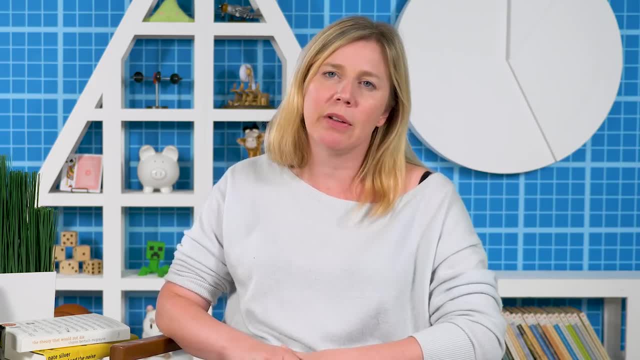 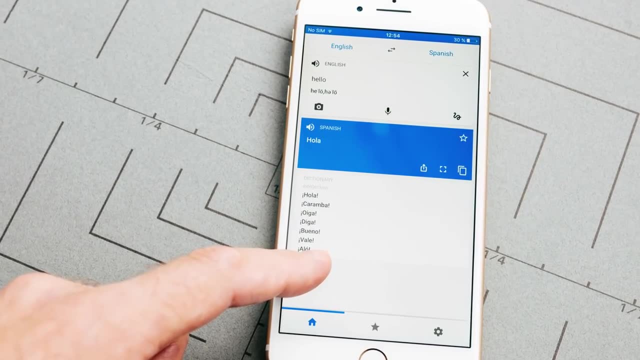 And while Bayesian inference is increasingly popular in many scientific fields like psychology, it's also being used right now in many places near you. Bayesian methods are used to help translate one language to another and to suggest which items you might buy next, based on the fact that you just bought four silicon sponges. 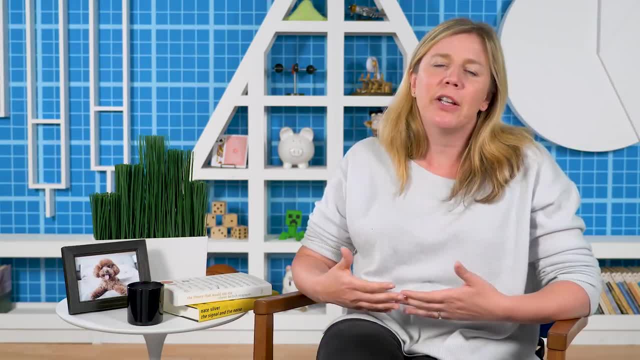 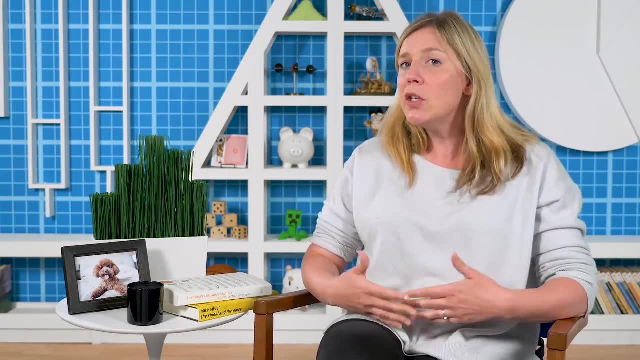 a sandalwood candle and a paper. Bayes can help you figure out which allergy medicine you'll react best to based on your genetic profile, And Bayes plays a role in creating artificial intelligence that can do pretty amazing things, Like understanding that it's more likely that you said Siri, turn on the lights and 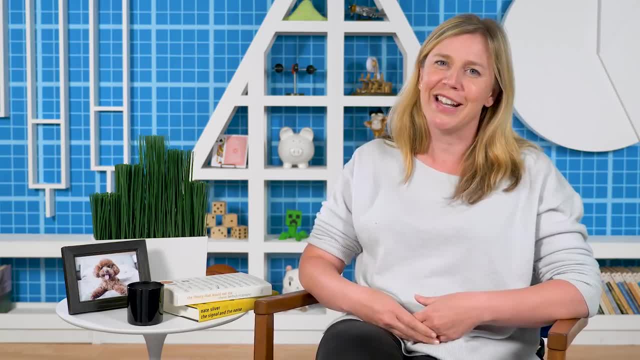 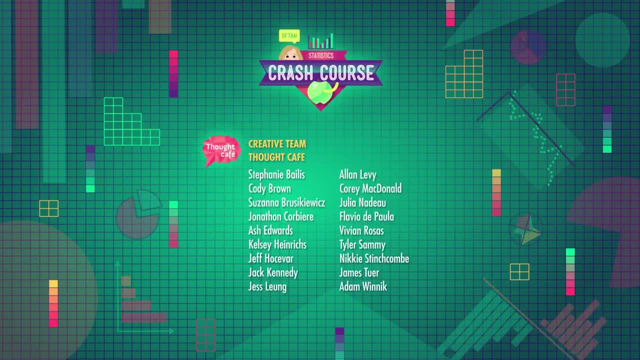 not Siri. learn all the sights. Thanks for watching. I'll see you next time. Crash Course Statistics is filmed in the Chad and Stacey Emigholz Studio in Indianapolis, Indiana, And it's made with the help of all these nice people.